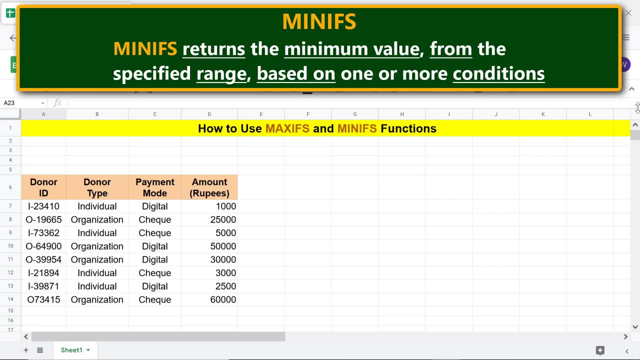 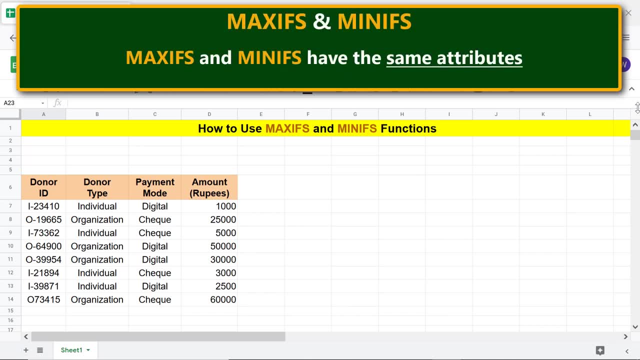 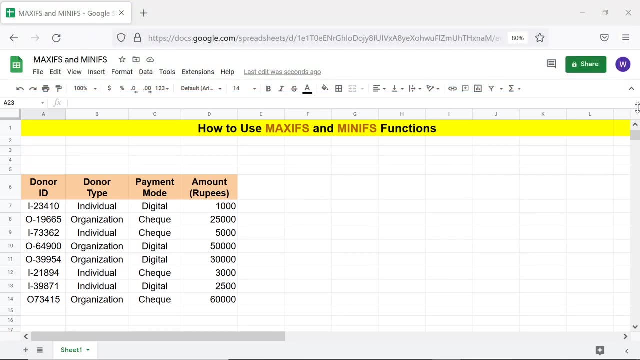 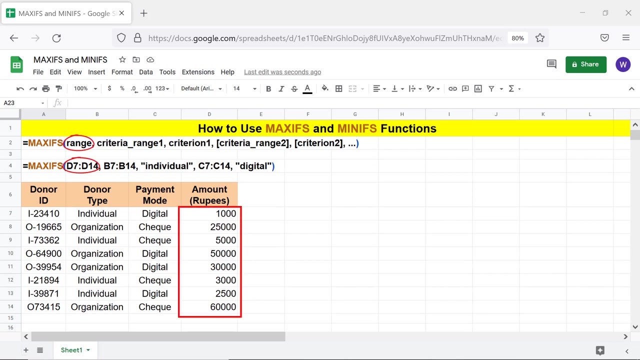 Minitifs returns the minimum value from the specified range based on one or more conditions. Maxifs and Minifs have the same attributes. Ok, let's look at the format of the Maxifs function formula. Here is an example. Range is a spreadsheet area from which to extract the maximum value. 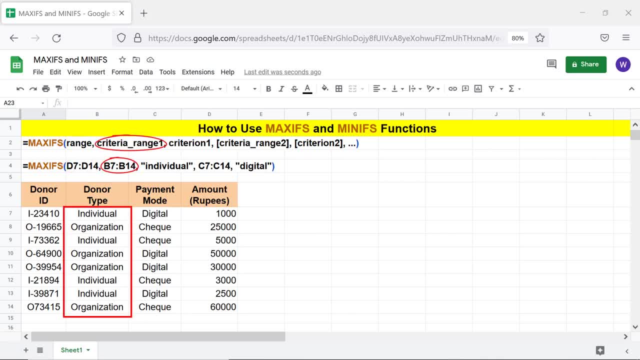 Criteria range 1 is a spreadsheet area which might have the value specified as criterion 1.. Criterion 1 is the first condition. Criteria range 2, criterion 2 and subsequent attributes are optional. The attributes and attribute description of Minifs are the same as that of Maxifs. 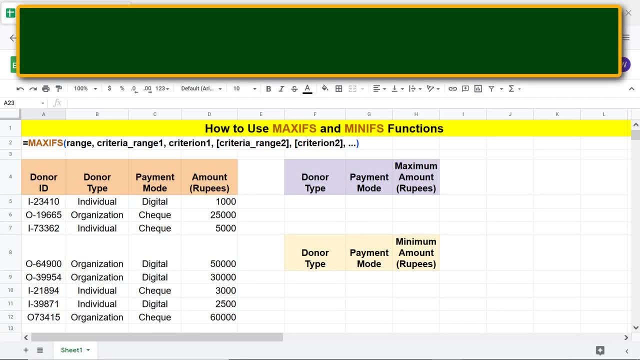 Going forward here is an objective of using Maxifs and Minifs To get the maximum and minimum donations, respectively, made by individuals or organizations through digital or check modes. I will type criterion 1,, which are the two donor types, and criterion 2,, which is a payment mode. 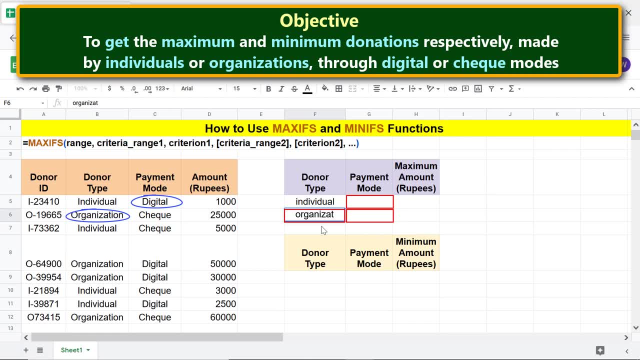 I will make this data display here by typing equal to and clicking the cell. I will make this data display here by typing equal to and clicking the cell. Alright, we are ready to type the Maxifs function formula here and Minifs function formula here. 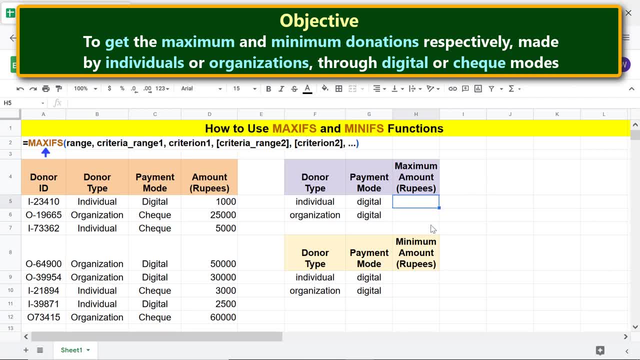 Let's start with Maxifs First type equal to M, A, X, I and select Maxifs For range. select this area. Type comma For criteria: range 1, select this range. Type comma For criterion 1, click this cell. 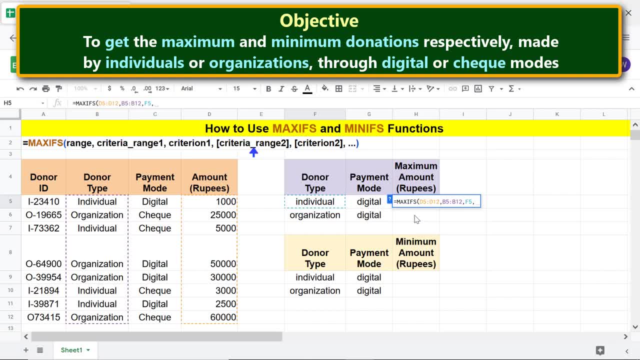 Type comma For criteria range 2, select this range. Type comma For criterion 2, click this cell. Type comma For criterion 2, click this cell. Type comma For criterion 2, click this cell. Press Enter. 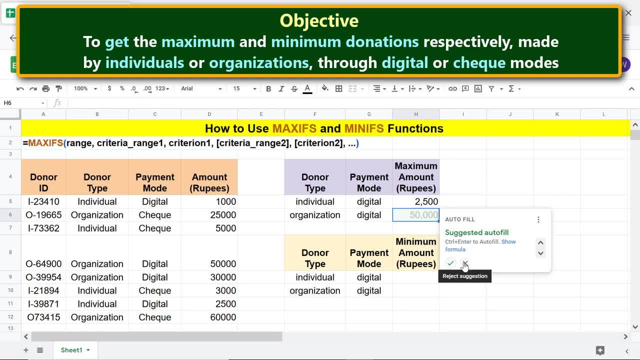 I will cancel auto fill because the output will not consider the correct ranges. We can simply copy this formula to this cell. However, we need to make the range- criteria range 1, and criteria range 2,- absolute. These do not change when we copy the formula. 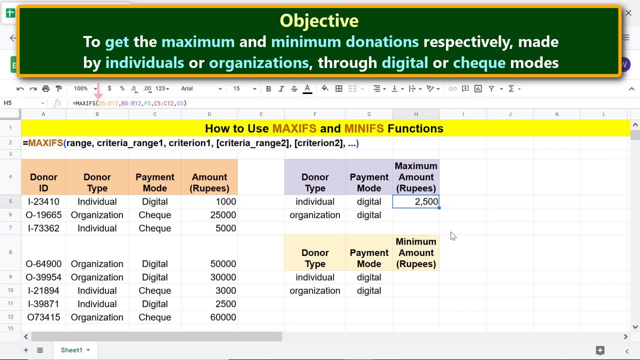 Click this cell. Click here and press F4.. Note that F4 is the key you have to press to make an address absolute. Press Enter, Copy the formula to this cell. There you go. These are the maximum donations received from individuals and organizations through. 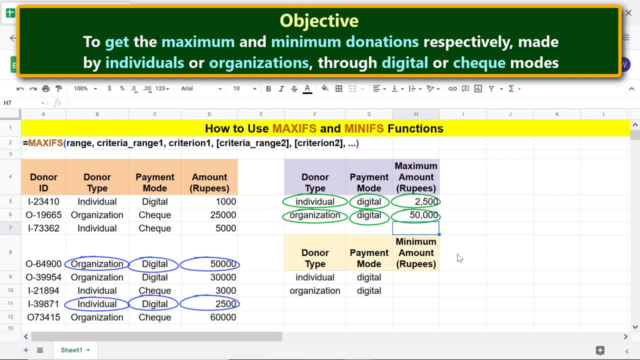 the digital mode To get the minimum values. first we need to simply copy the formula in this cell to this cell. Next, change the function name to Minifs, Press Enter. Autofill the cell. All right, here are the minimum values. 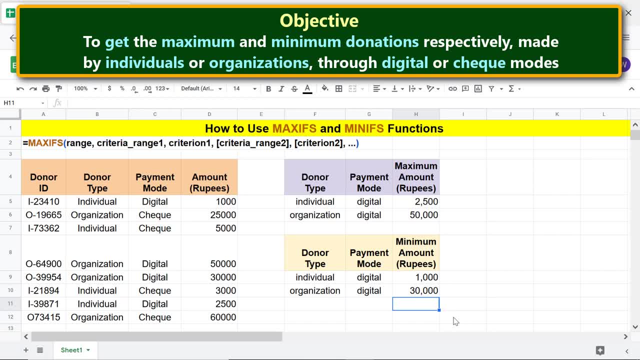 If you wish to get the maximum and minimum donations, you can click here, And if you want to get the minimum values left, just hold down the mouse key. for example, The value you want to get is now confused. Is it going to fit the change? 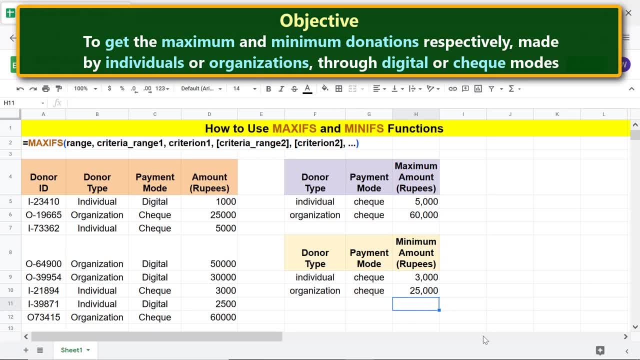 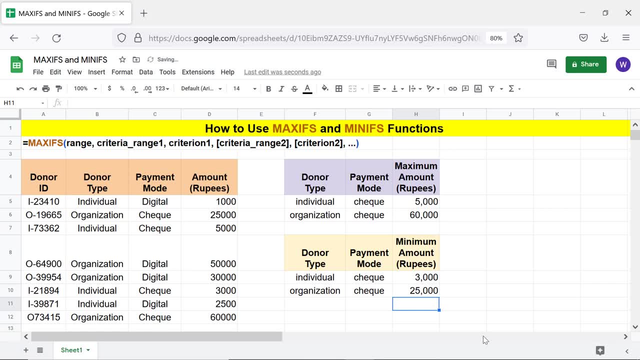 All you have to do is Change the value for criterion 2.. That's it, folks. Thank you for watching this video. Please subscribe to this channel.